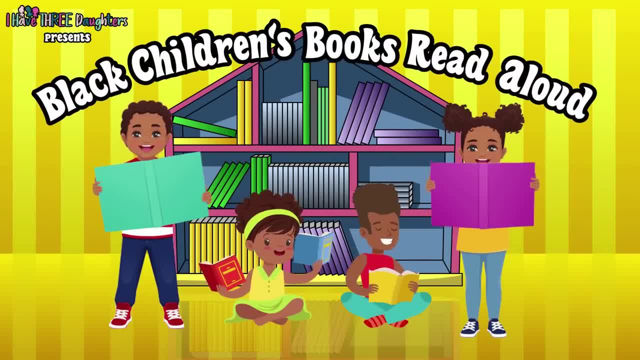 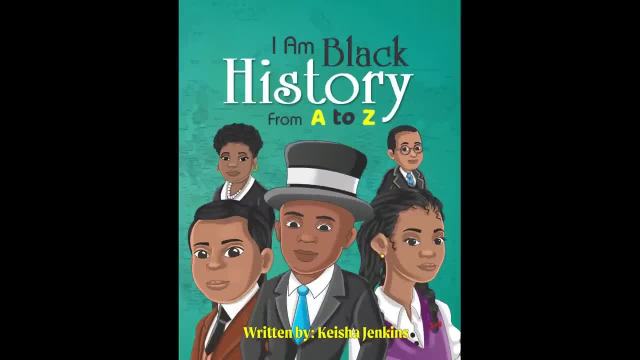 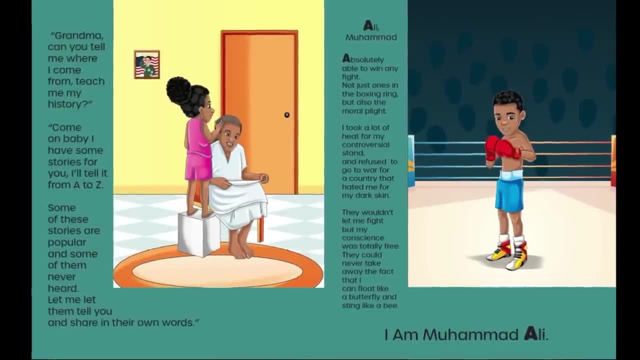 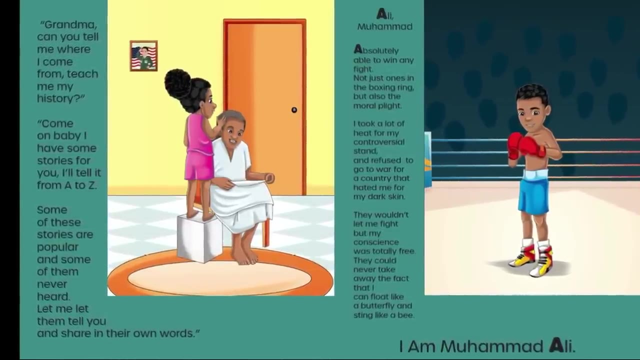 Welcome to Black Children's Books. Read Aloud: I am Black. History from A to Z written by Keisha Jenkins. Grandma, can you tell me where I come from? Teach me my history. Come on, baby, I have some stories for you. I'll tell you from A to Z. 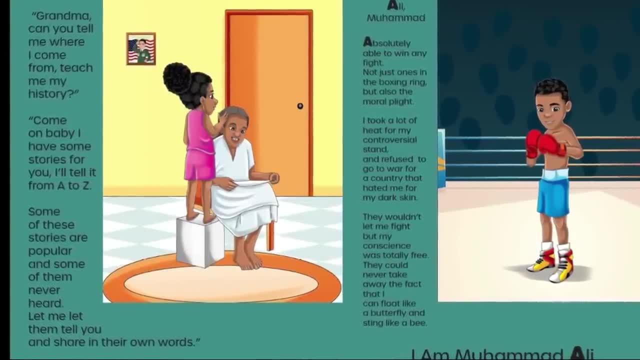 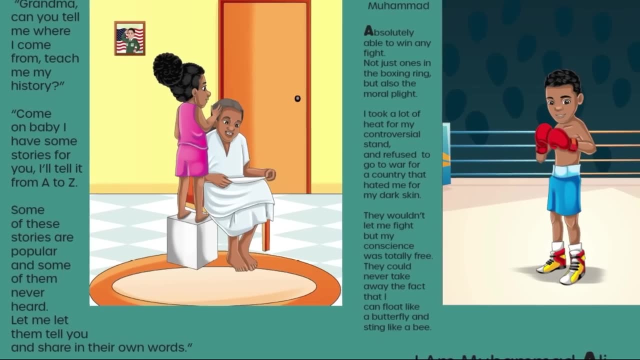 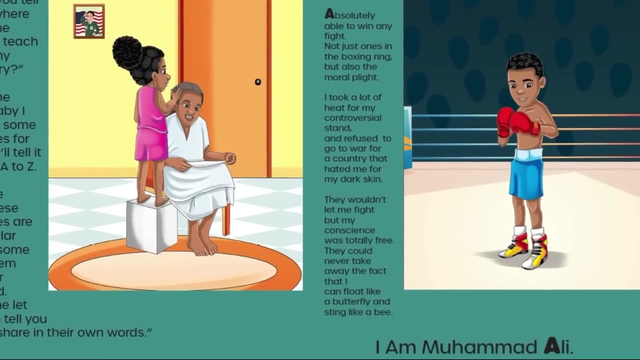 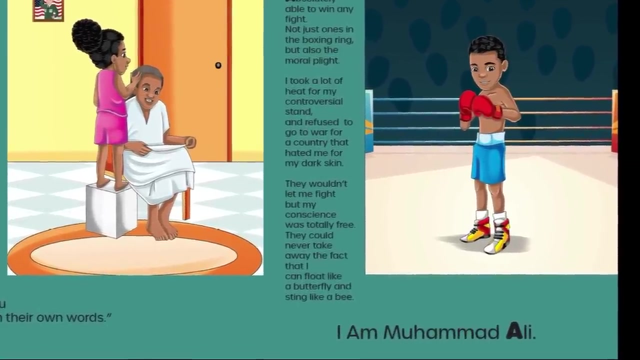 Some of these stories are popular and some never heard. Let me let them tell you and share in their own words. Muhammad Ali: Absolutely able to win any fight, Not just once the boxing ring, but also the moral plight. I took a lot of heat from my controversial stand and refused to go to war for a country that hated me for my dark skin. 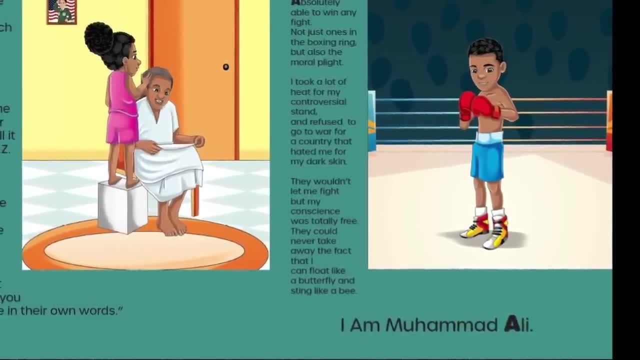 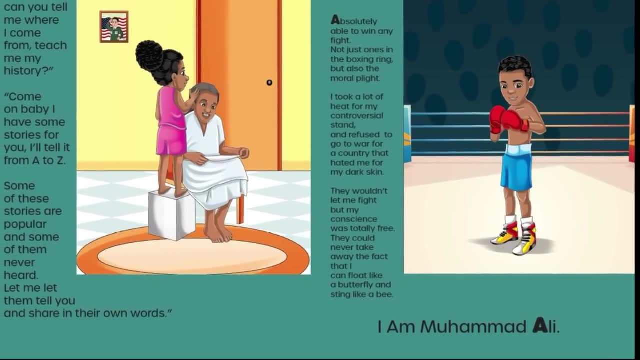 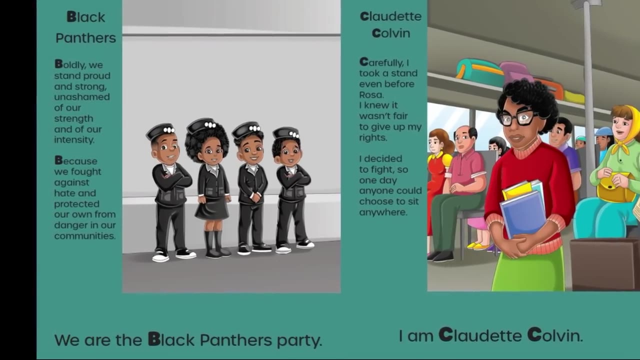 They wouldn't let me fight, but my conscience was totally free. They could never take away the fact that I can float like a butterfly and sting like a bee. I am Muhammad Ali Black Panthers. Boldly, we stand, proud and strong, unashamed of our strength and our intensity. 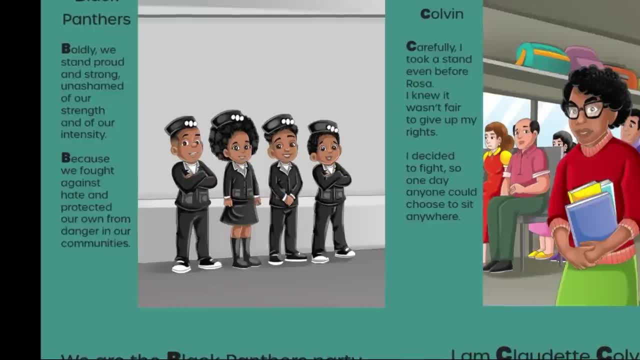 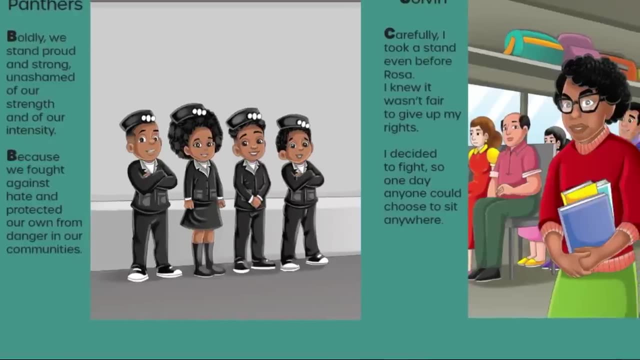 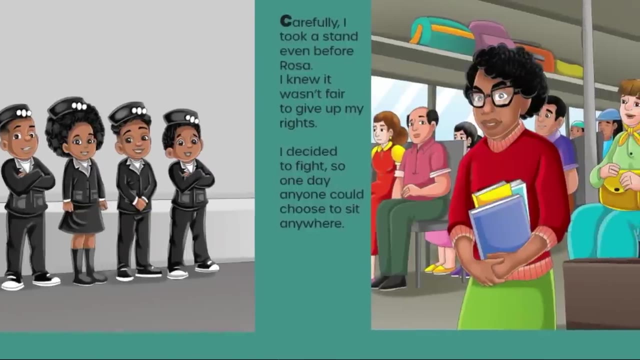 because we fought against hate and protected our own from dangers in our communities. We are the Black Panthers Party. Claudette Colvin. Carefully, I took a stand even before Rosa. I knew it wasn't fair to give up my rights. I decided to fight so one day anyone could choose to sit anywhere. 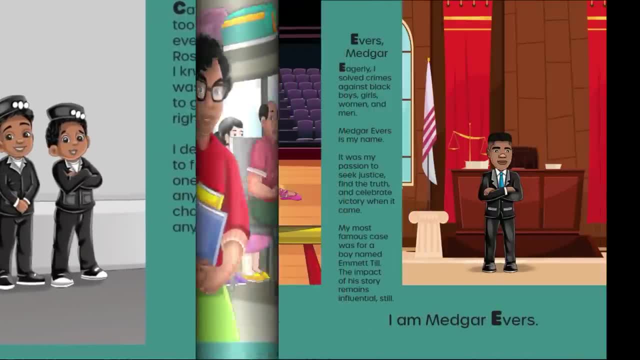 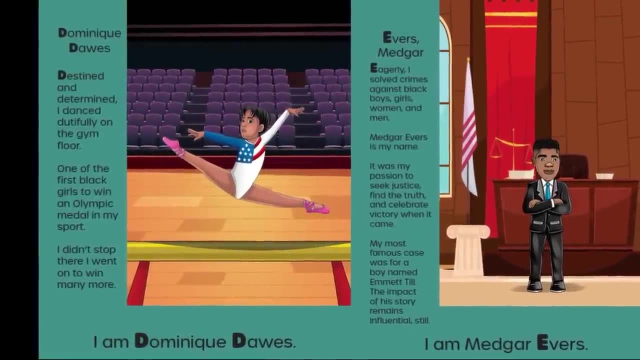 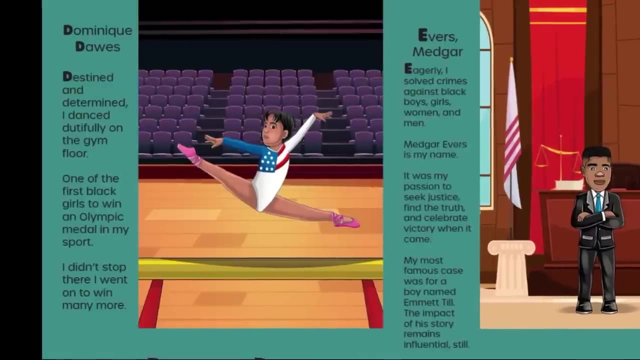 I am Claudette Colvin, Dominique Dawes. Destined and determined, I danced dutifully on the gym floor, One of the first black girls to win an Olympic medal In my sport. I didn't stop there. I went on to win many more. 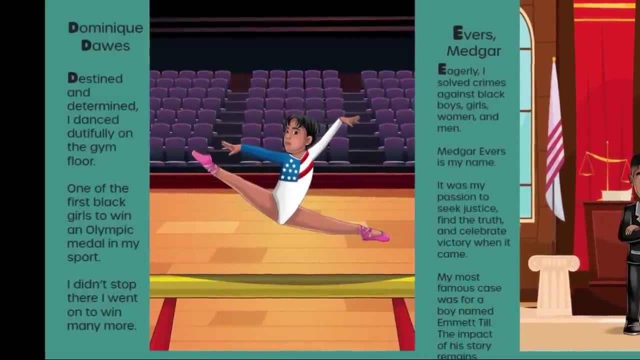 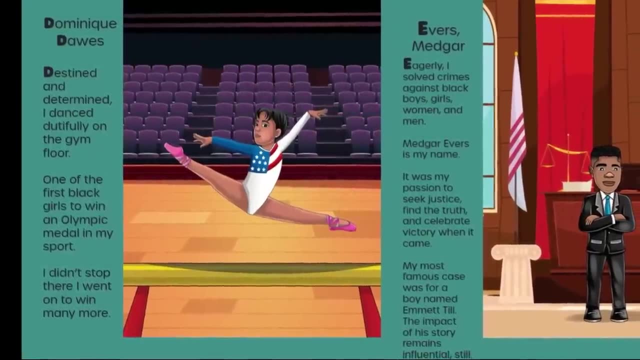 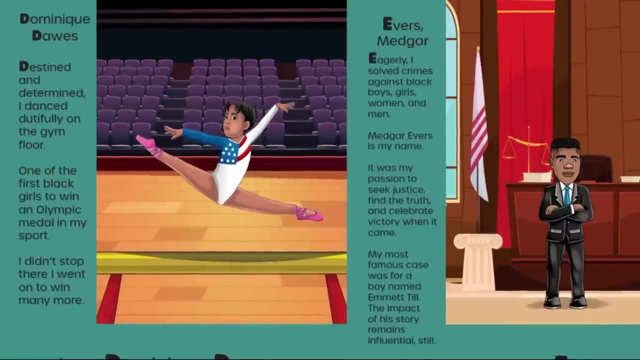 I am Dominique Dawes Megger Evers. Eagerly I solved crimes against black boys, girls, women and men. Megger Evers is my name. It was my passion to seek justice, find the truth and celebrate victory when it came. 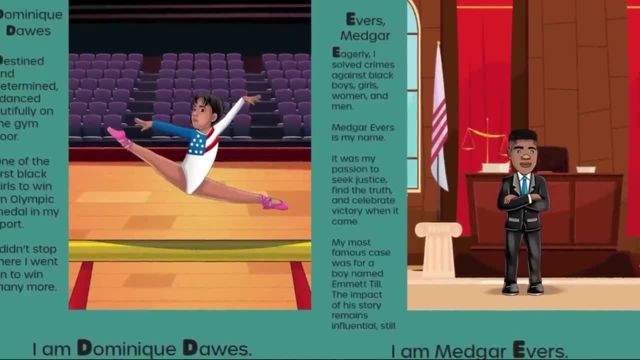 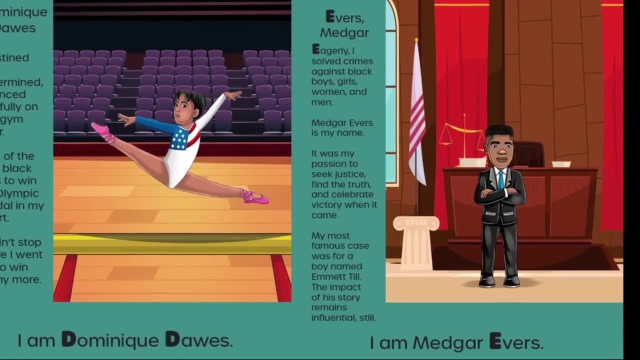 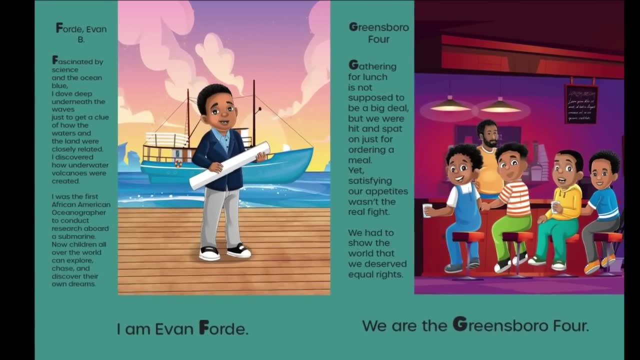 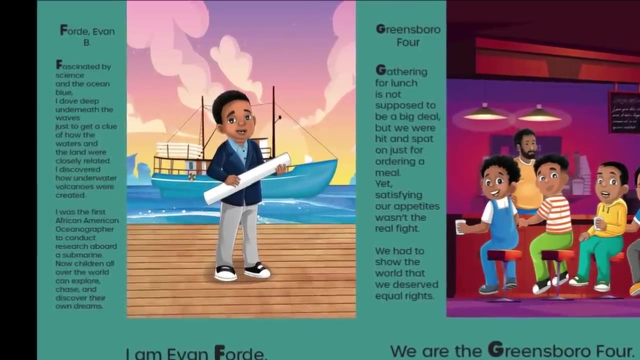 He was a black man. The impact of his story remains influential still. I am Megger Evers, Evan B Ford. Fascinated by science and the ocean blue, I dug deep underneath the waves just to get a clue of how the waters and the land were closely related. 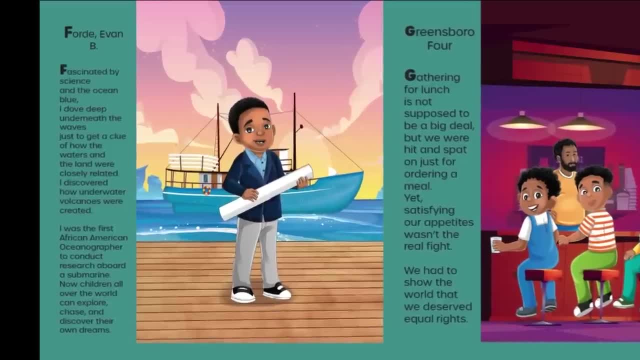 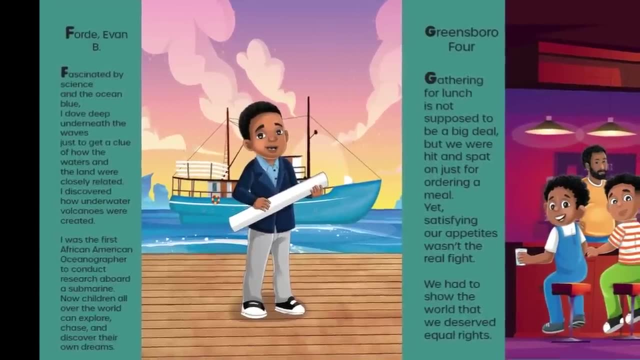 I discovered how underwater volcanoes were created. I was the first African American oceanographer. I was the first African American oceanographer to conduct research aboard a submarine. I was the first African American oceanographer to conduct research aboard a submarine. I was the first African American oceanographer to conduct research aboard a submarine. 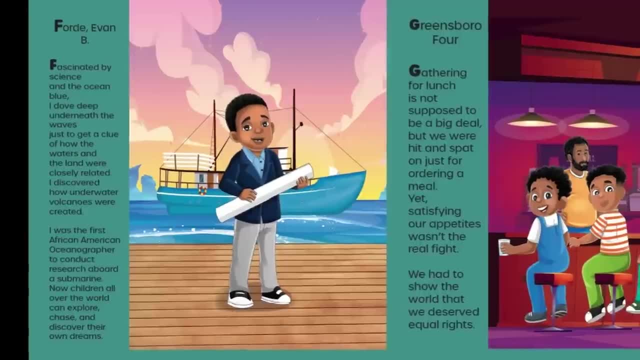 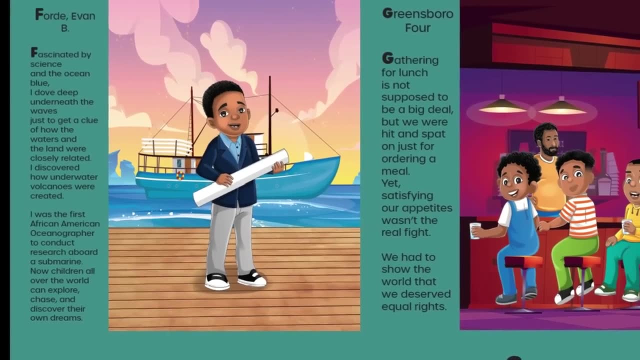 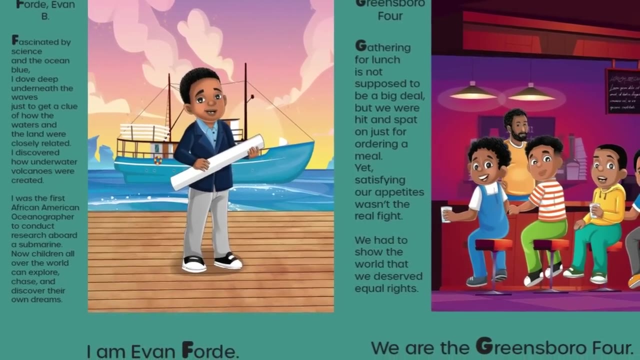 New children all over the world can explore, chase and discover their own dreams. I am Evan Ford, Greensboro 4. Gathering for lunch is not supposed to be a big deal, but we were hit and spat on just for ordering a meal. 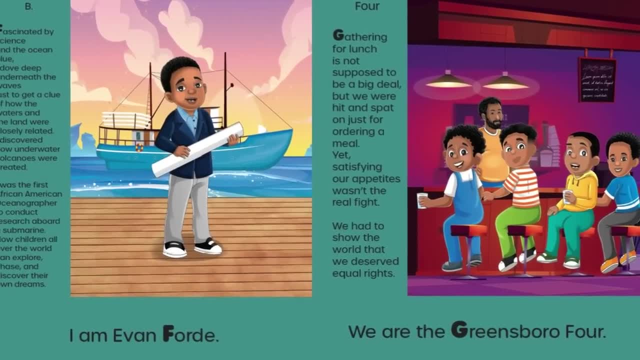 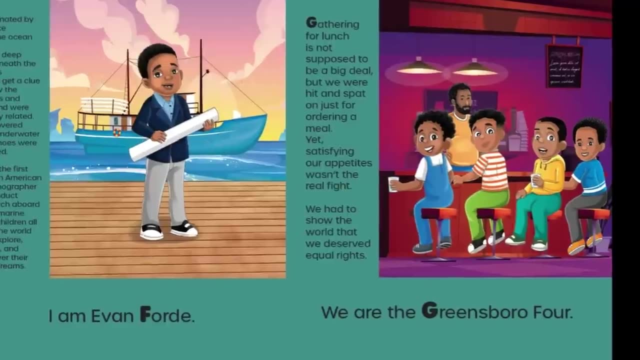 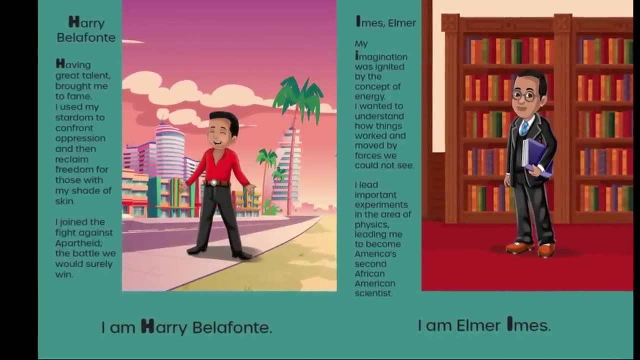 Yet satisfying our appetites wasn't the real fight. We had to show the world- We had to take a big bite- that we deserved equal rights. We are the Greensboro Four. Harry Belafonte, Having great talent, brought me to fame. 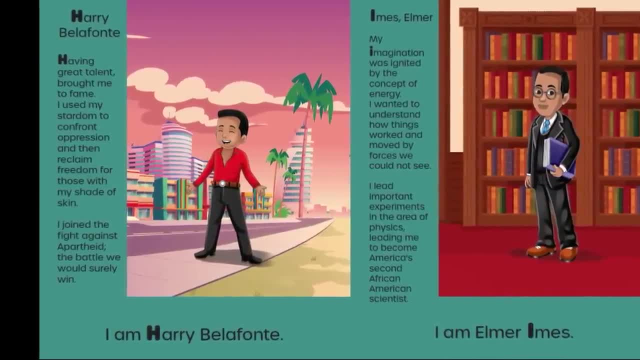 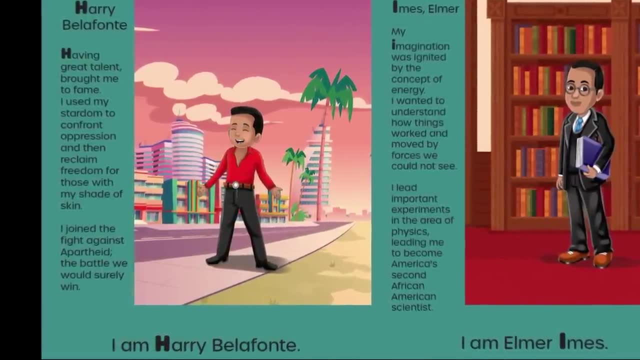 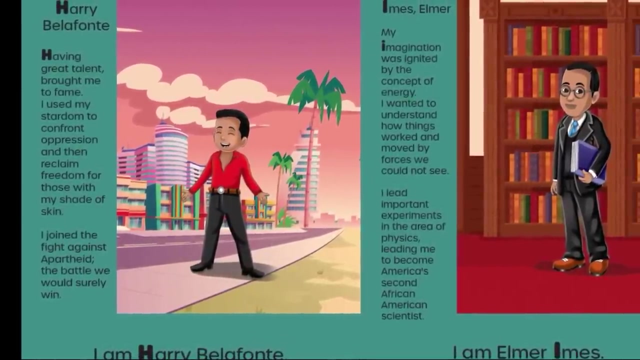 I used my stardom to confront oppression and then reclaim freedom for those with my shade of skin. I joined the fight against apartheid, but battle we'd surely win. I am Harry Belafonte, Elmer Imes. My imagination was ignited by the concept of energy. 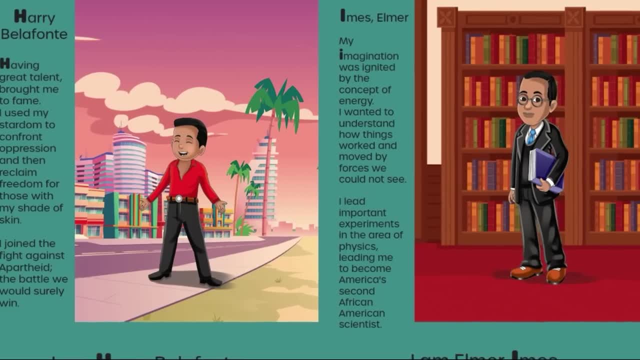 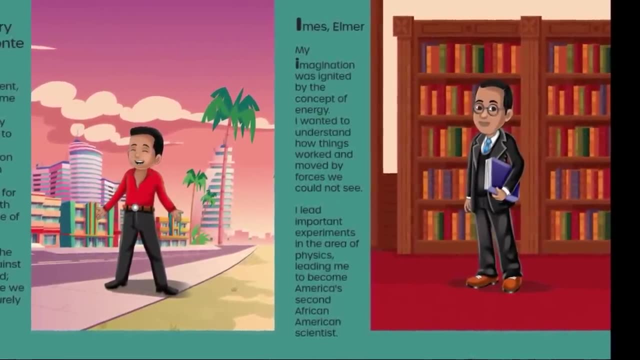 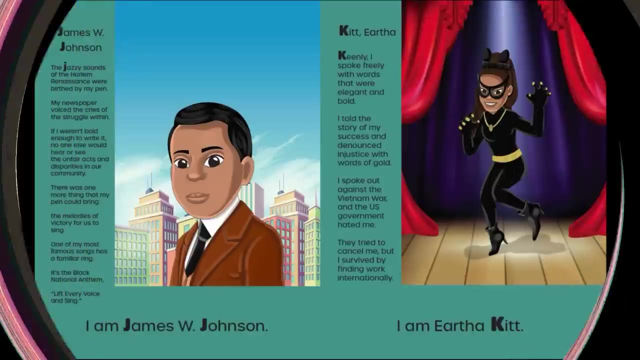 I wanted to understand how things worked and moved by forces we could not see. I led important experiments in the area of physics, leading me to become America's second African-American scientist. I am Elmer Imes. James W Johnson. The jazzy sounds of the music. 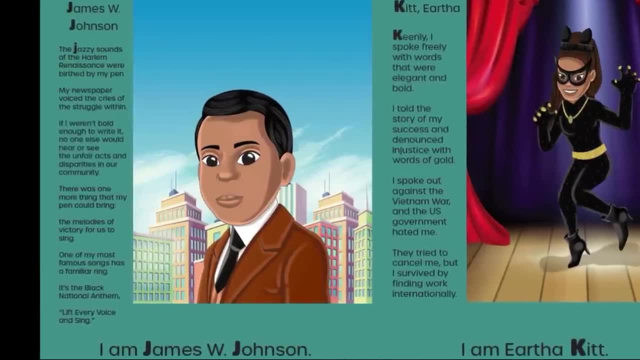 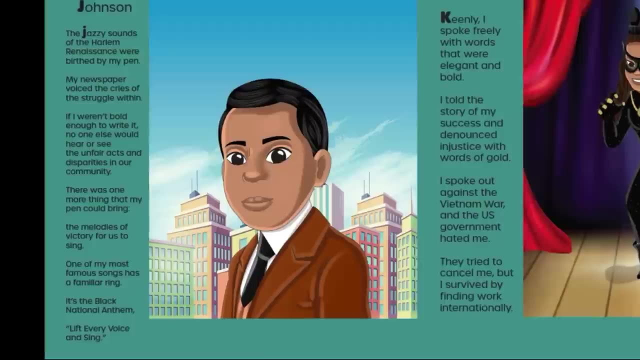 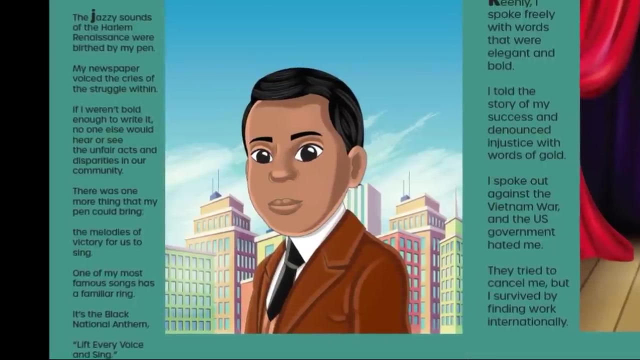 of the Harlem Renaissance were birthed by my pen. My newspaper voiced the cries of the struggle within. If I weren't bold enough to write it, no one else would hear or see the unfair acts of disparities in our community. There was one more thing that my pen could bring. 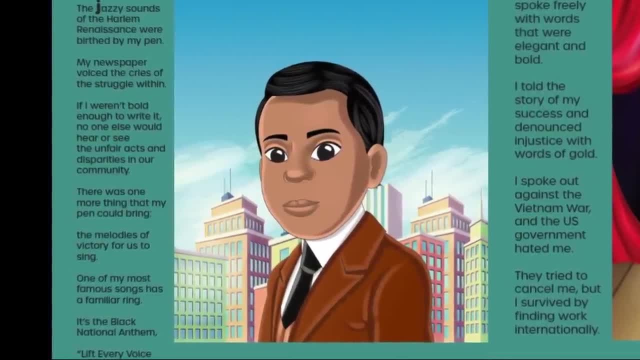 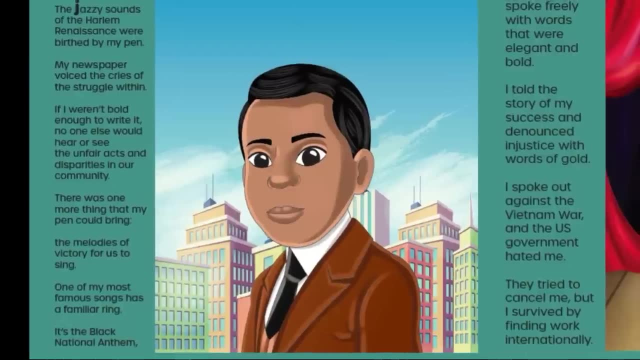 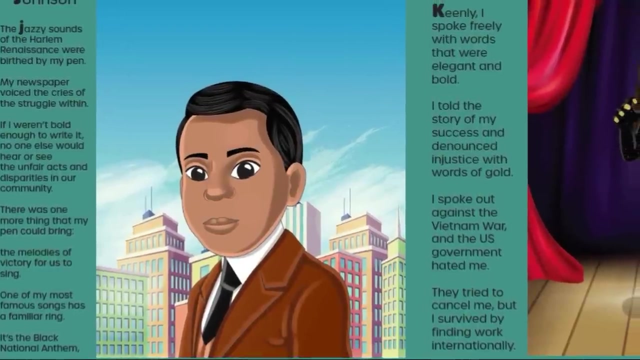 the melodies of victory for us to sing. One of my most famous songs has a familiar ring. It's the Black National Anthem. Lift every voice and sing. I am James W Johnson, Eartha Kitt Keenly. I spoke freely, with words that were elegant and bold. 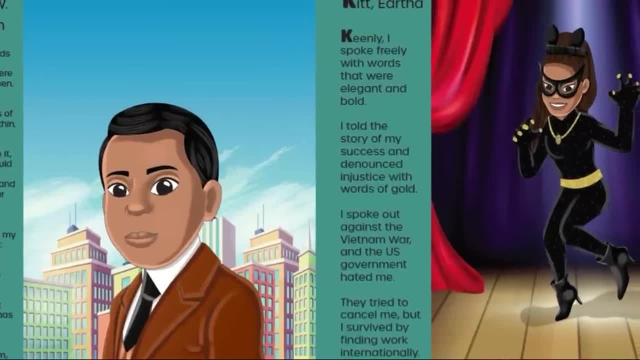 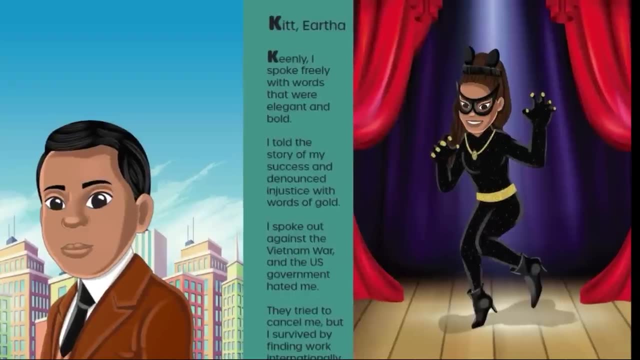 I told the story of my success in denouncing justice with words of gold. I spoke out against the Vietnam War and the US government hated me. They tried to cancel me, but I survived by finding work internationally. I am Eartha Kitt. 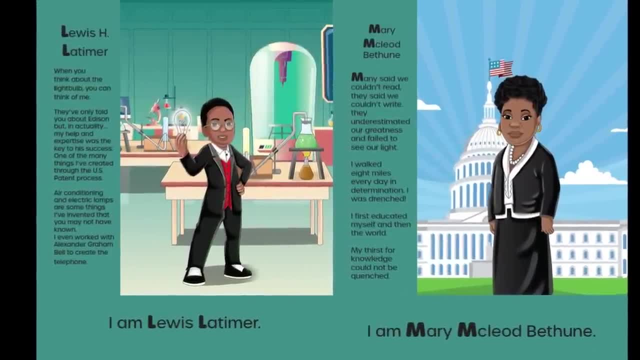 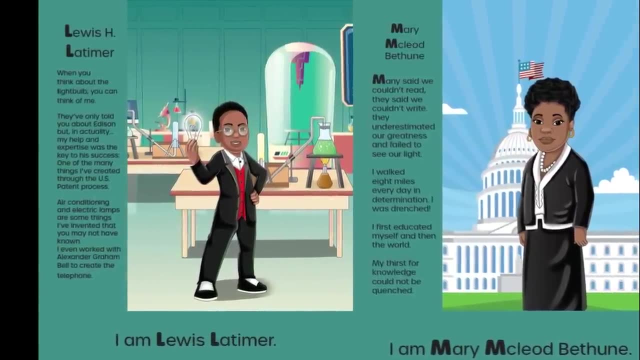 Lewis H Latimer, When you think about the light bulb, you can think of me. They've only told you about Edison, but in actuality, my help and expertise was the key to his success- one of the many things I've created. 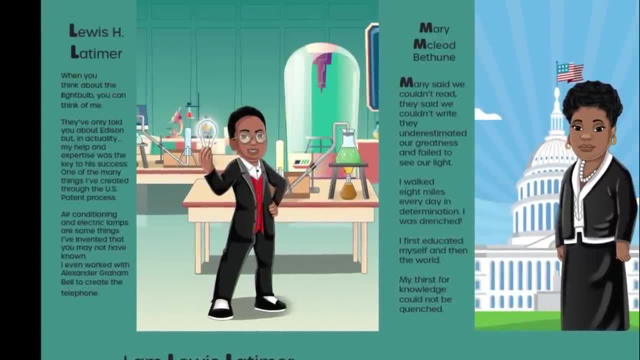 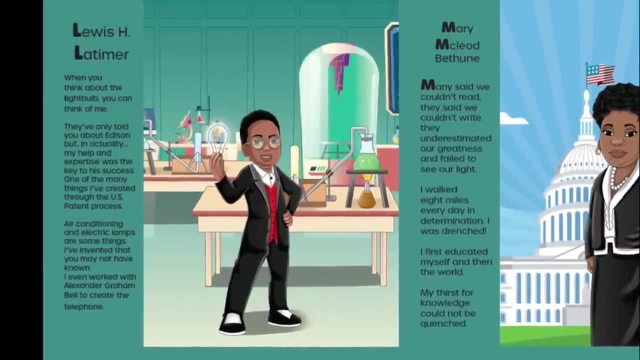 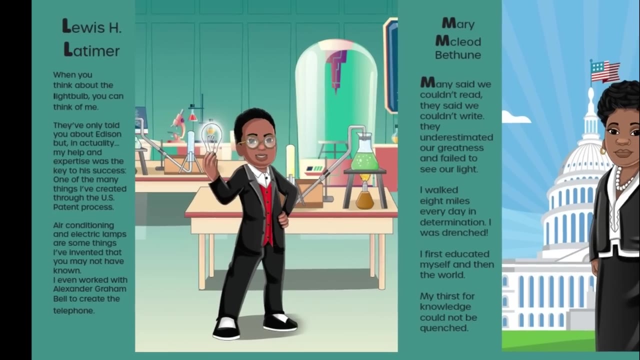 through the US patent process. Air conditioning and electric lamps are some things I've invented that you may not have known. I even worked for Alexander Graham Bell to create the telephone. I am Lewis Latimer, Mary McLeod Bethune. Many said we couldn't read. 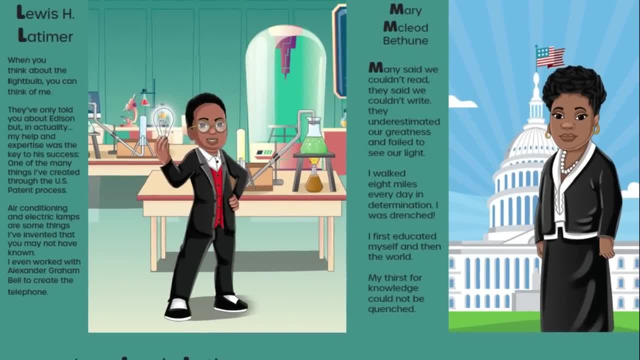 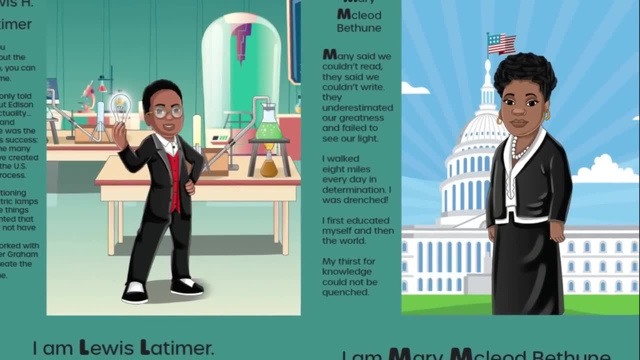 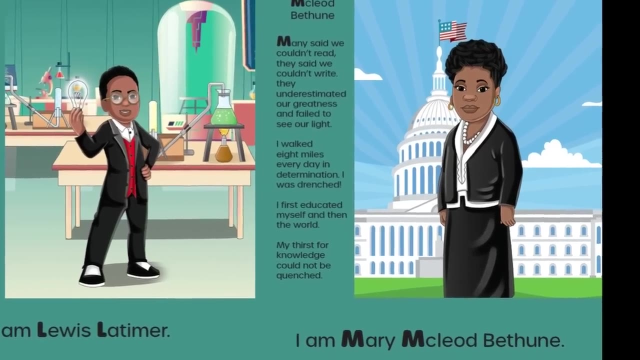 They said we couldn't write. They underestimated our greatness and failed to see our light. I walked eight miles every day in determination. I was drenched. I first educated myself and then the world. My thirst for knowledge could not be quenched. 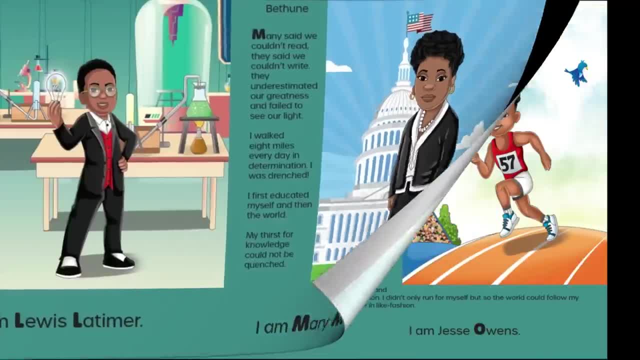 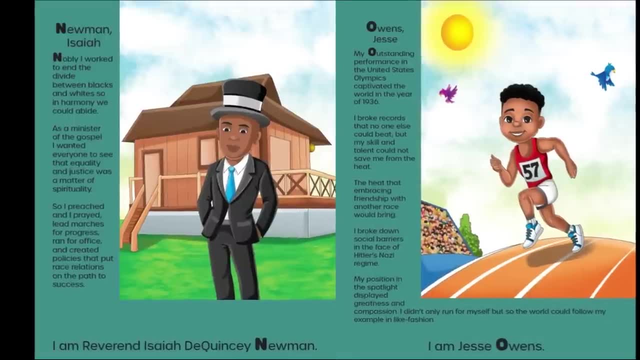 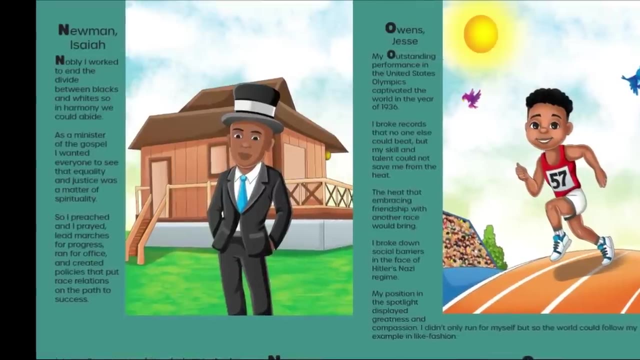 I am Mary McLeod, Bethune, Isaiah Newman Nobly. I worked to end the divide between blacks and whites so in harmony we could abide. As a minister of the gospel, I wanted everyone to see that equality and justice was a matter of spirituality. 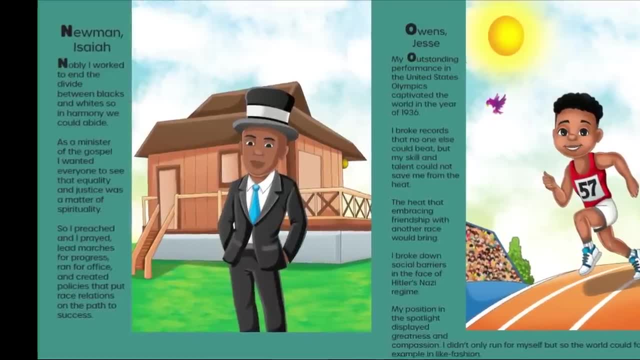 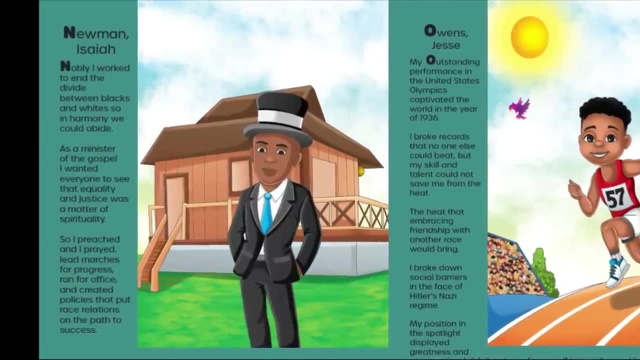 So I preached and I prayed, led marches for progress, ran for office and created policies that put race relations on the path to success. I am Reverend Isaiah DeQuincey Newman. I am Reverend Isaiah DeQuincey Newman. 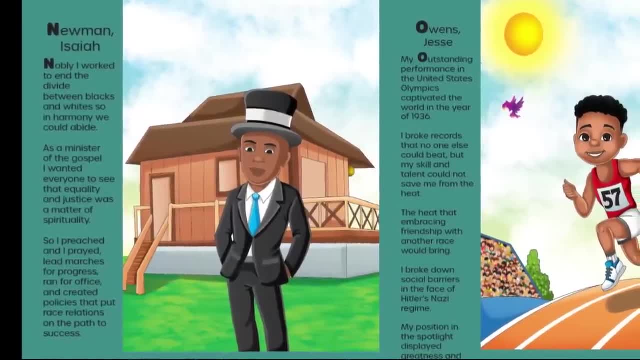 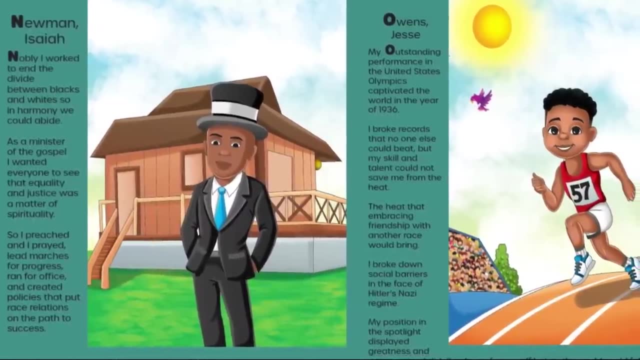 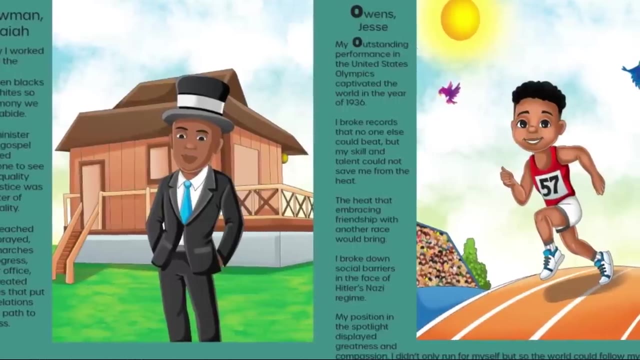 Jesse Owens. My outstanding performance in the United States Olympics captivated the world in the year of 1936. I broke records that no one else could beat, but my skill and talent could not save me from the heat, The heat that embracing friendship. 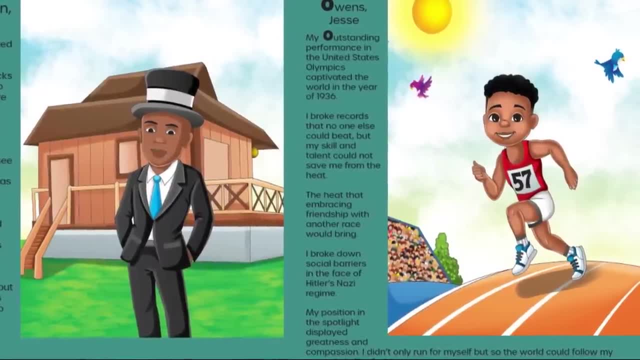 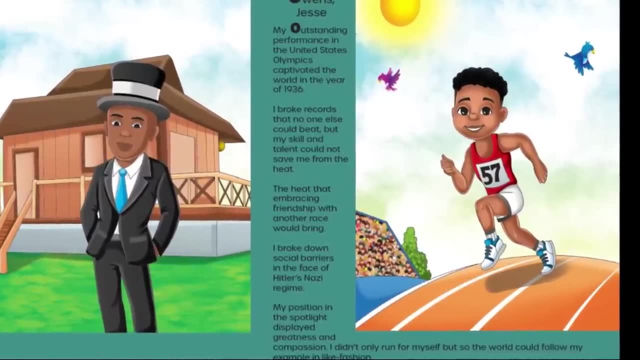 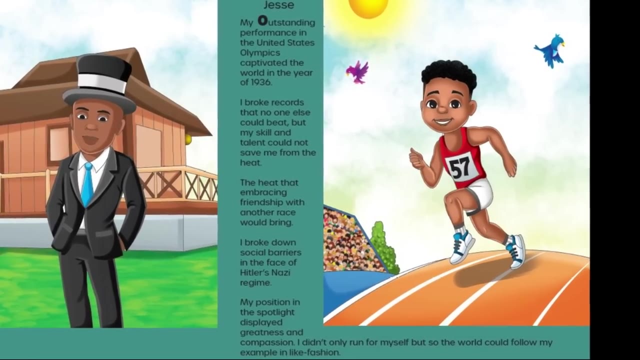 with another race would bring. I broke down social barriers in the face of Hitler's Nazi regime. My position in the spotlight displayed greatness and compassion. I didn't only run for myself, but so the world could follow my example in like fashion. I am Jesse Owens. 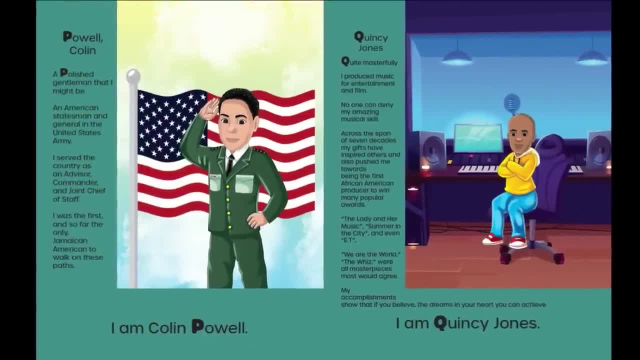 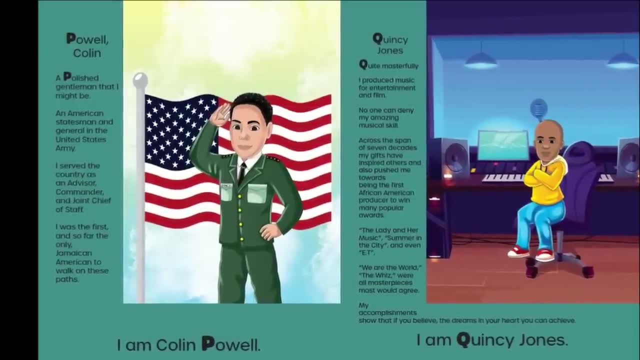 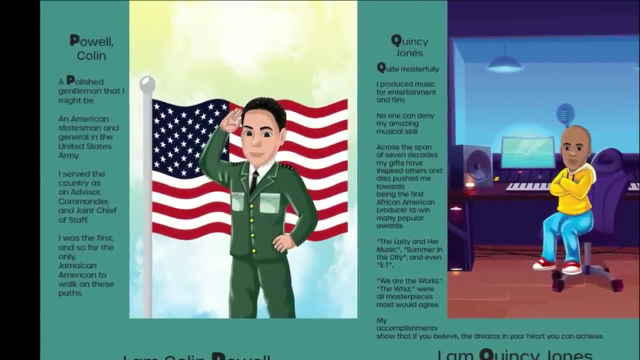 I am Jesse Owens Colon Powell, A polished gentleman that I might be an America statesman and general in the United States Army. I served the country as an advisor commander and joint chief of staff. I was the first and so far the least. to ever be the world's greatest fighter. I served the country as an advisor, commander and joint chief of staff. I was the first and so far the least the inspection effort to both participate in the fighting as the World's best fighter that collided its adults. 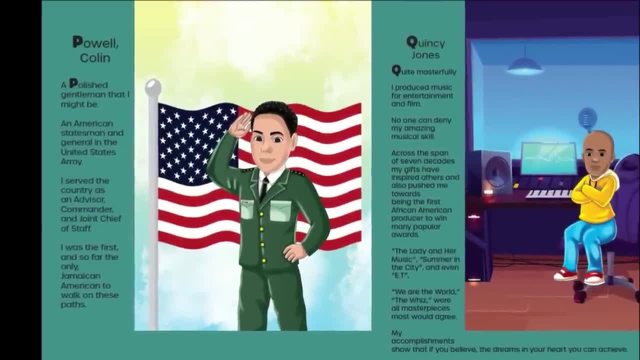 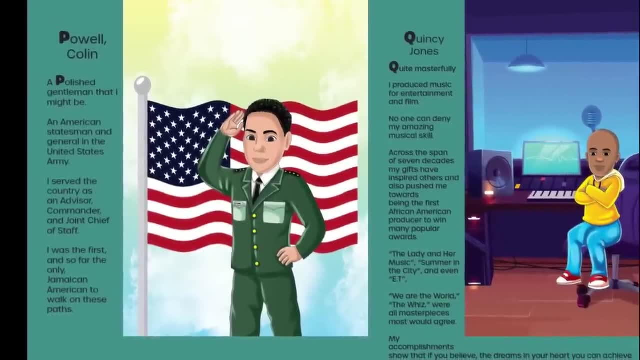 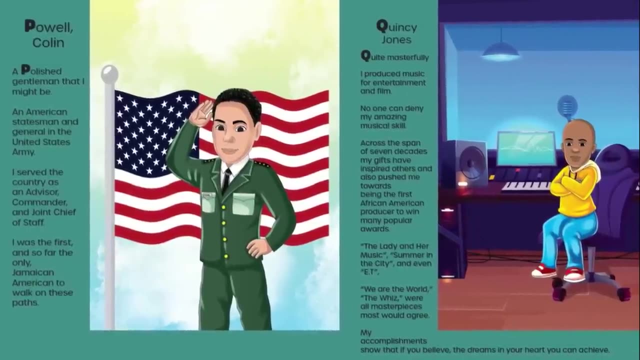 the only Jamaican American to walk on these paths. I am Colin Powell, Quincy Jones. Quite masterfully, I produce music for entertainment and film. No one can deny my amazing musical skill. Across the span of seven decades, my gifts have inspired others and also pushed me towards. 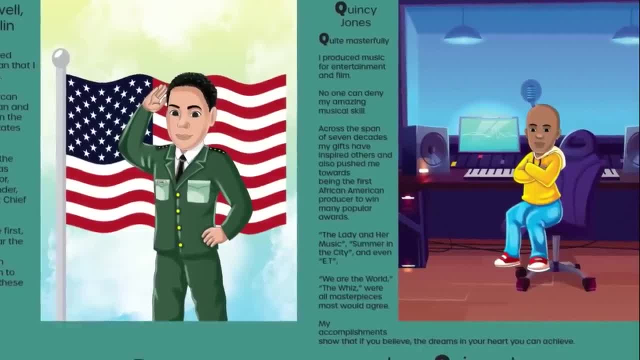 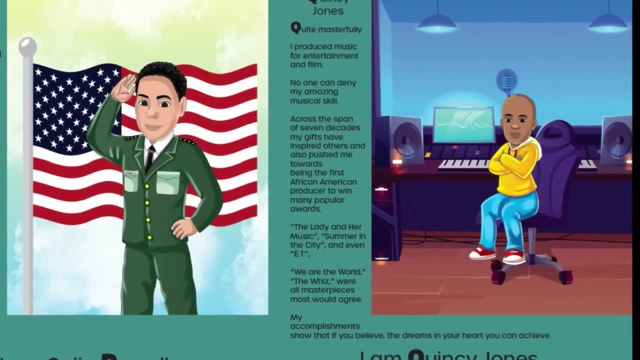 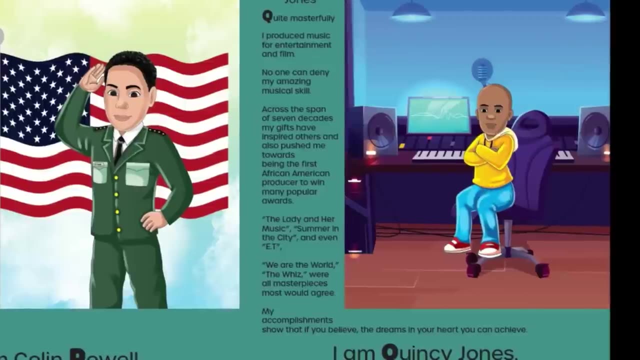 being the first African American producer to win many popular awards: The lady and her music, summer in the city and even ET. We are the world, the Wiz, we're all masterpieces. most would agree. My accomplishments show that, if you believe. 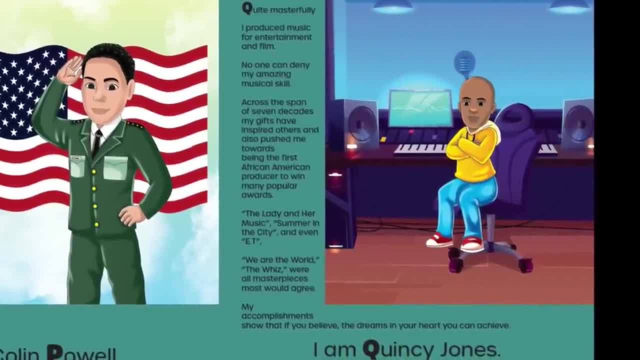 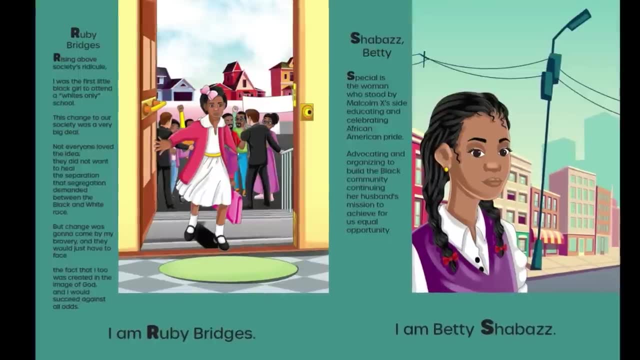 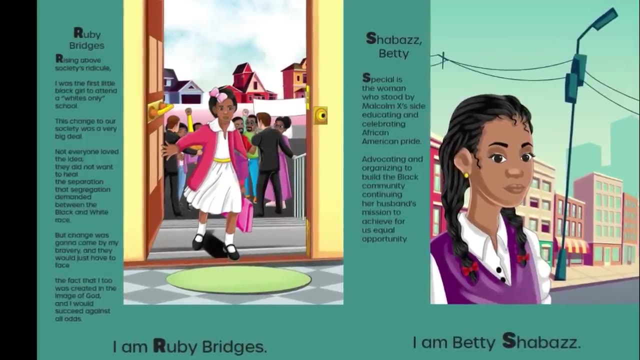 the dreams in your heart you can achieve. I am Quincy Jones Ruby Bridges, Rising above society's ridicule. I was the first black girl to attend a whites-only school. This change to our society was a very big deal. Not everyone loved the idea. they did not want to heal. 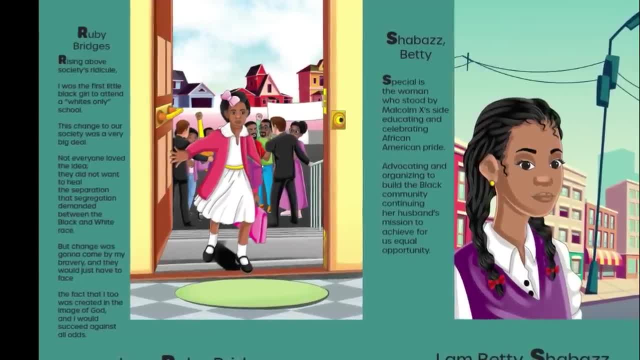 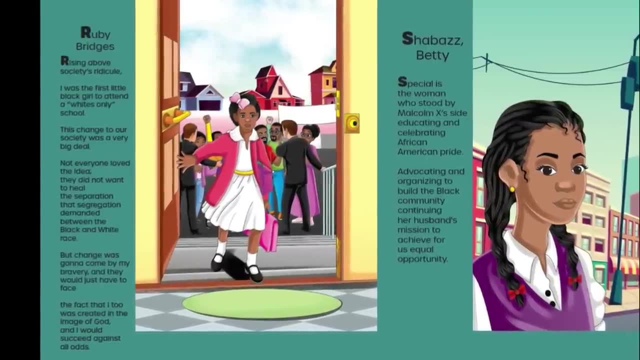 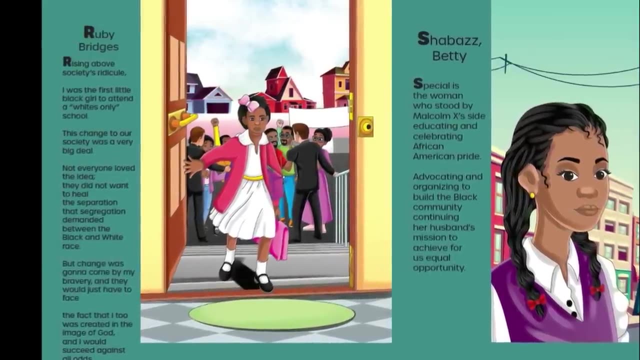 The separation, the segregation demanded between the black and white race. But change was gonna come by my bravery, and they would just have to face The fact that I too was created in the image of God and I would succeed against all odds. I am Ruby Bridges. 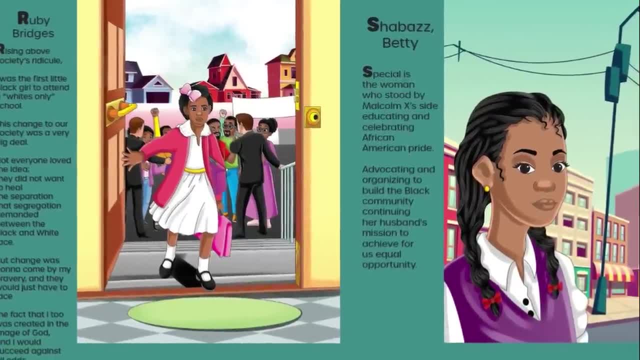 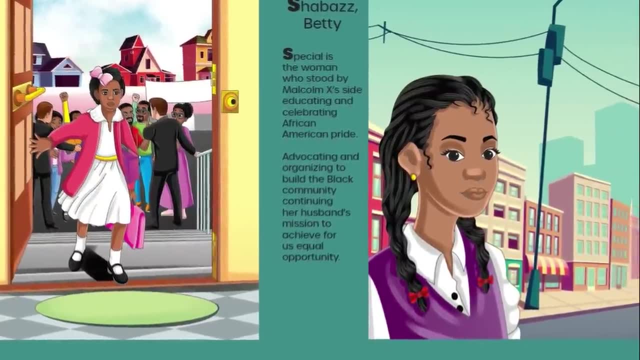 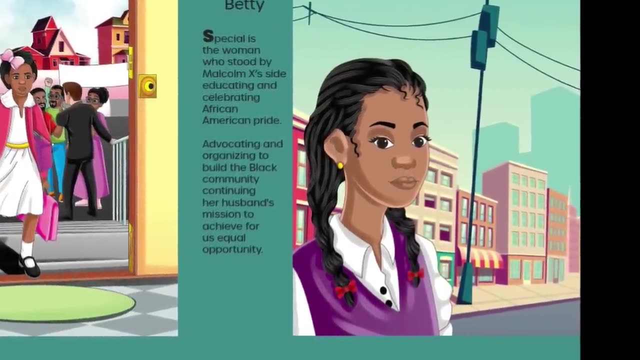 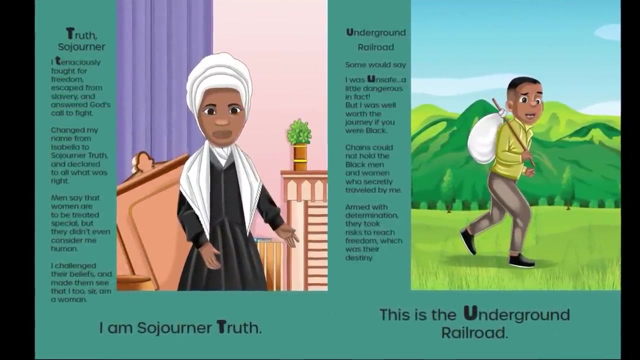 Betty Chavez Special is the woman who stood Malcolm X's side, educating and celebrating African American pride, Advocating and organizing to build the black community, continuing her husband's mission to achieve for us equal opportunity. I am Betty Chavez, Sojourner Truth. 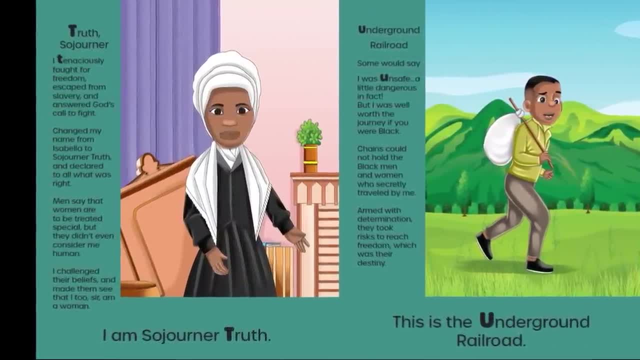 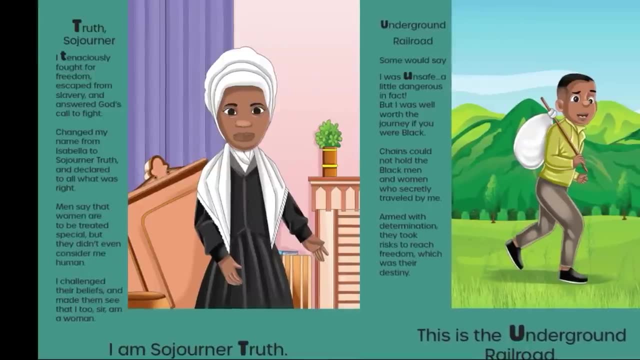 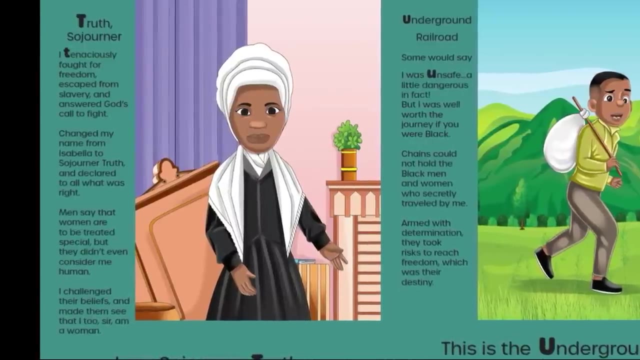 I tenaciously fought for freedom, escaped from slavery and answered God's call to fight, Changed my name from Isabella to Sojourner Truth and declared to all what was right. Men say that women are to be treated special, but they didn't even consider me human. 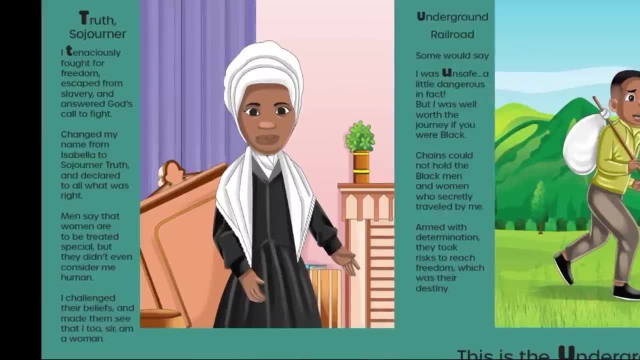 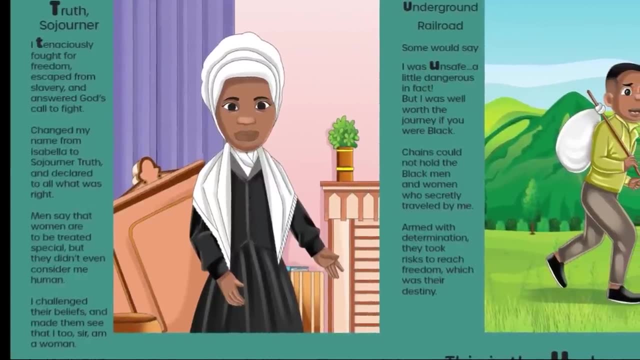 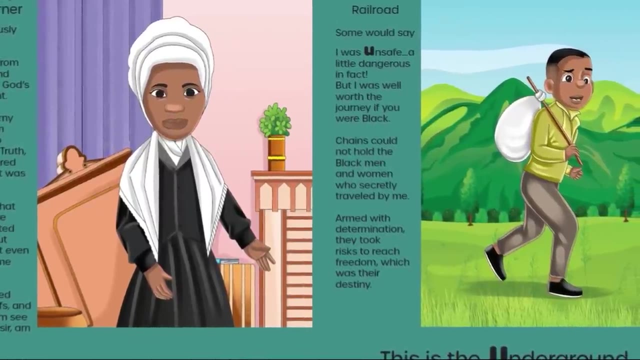 I challenged their beliefs and made them see that I too, sir, am a woman. I am Sojourner Truth. Underground Railroad. Some would say I was unsafe, a little dangerous in fact, but I was well worth the journey. if you were black. 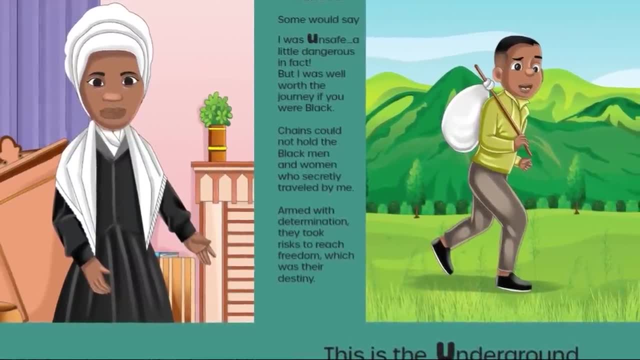 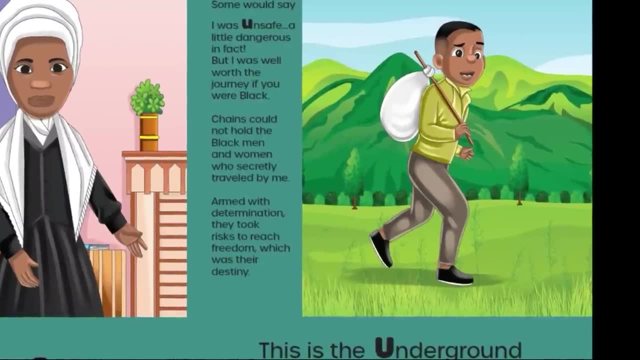 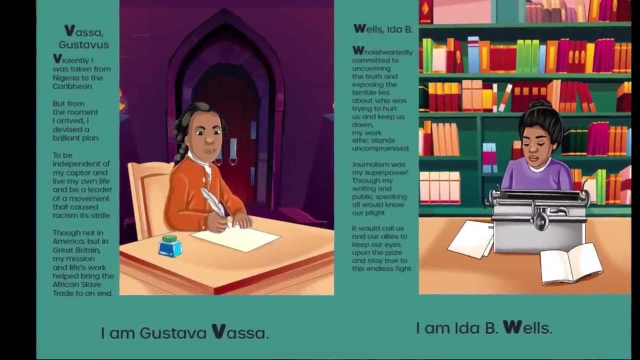 Chains could not hold the black men and women who secretly traveled by me. Armed with determination, they took risks to reach freedom, which were their destiny. This is the Underground Railroad: Gustavus Vassa. Violently, I was taken from Nigeria to the Caribbean. 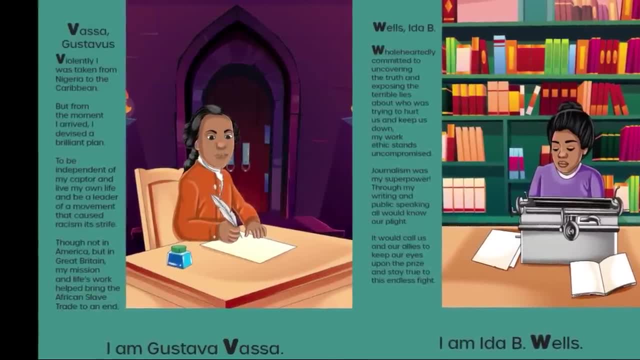 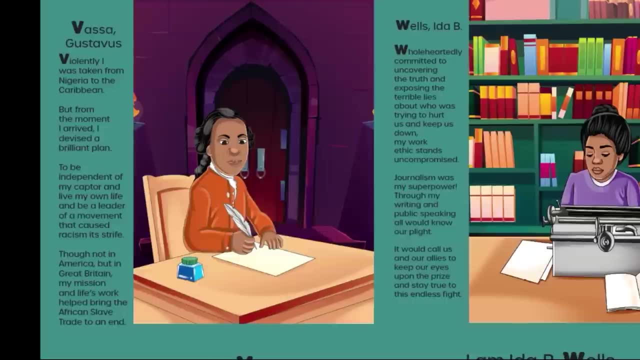 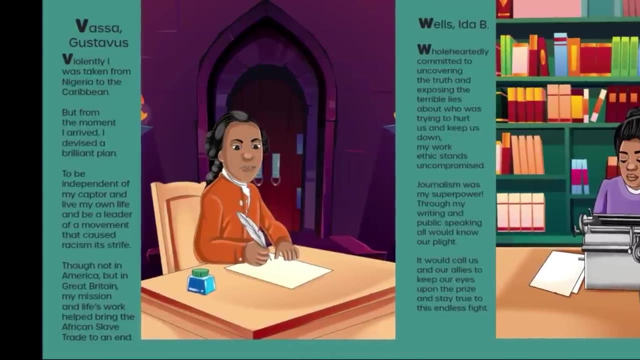 but from the moment I arrived, I devised a brilliant plan to be independent from my captor and live my own life and be a leader of a movement that calls racism is strife, Though not in America, but in Great Britain. my mission and life's work helped bring. 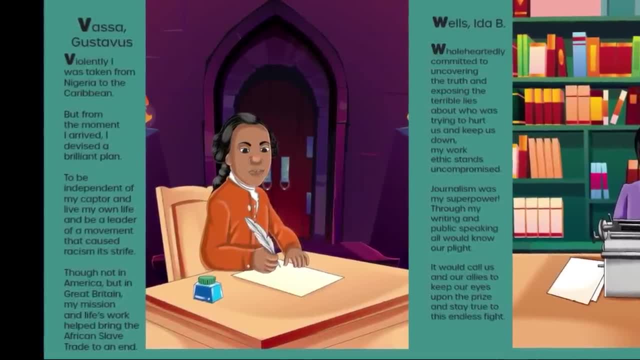 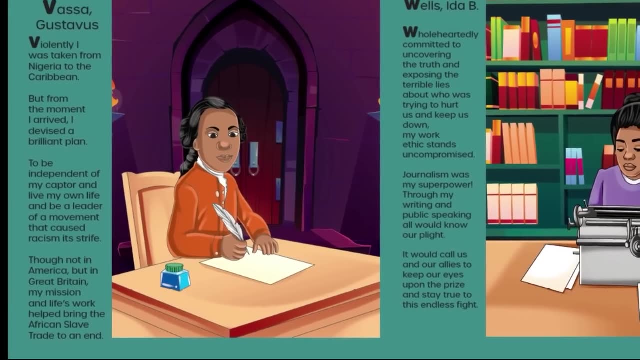 the American slave trade to an end. I am, Gustavus Vassa, Ida B Wells, Wholeheartedly committed to uncovering the truth and exposing the terrible lie about who was trying to hurt us and keep us down. my work ethics stand uncompromising. 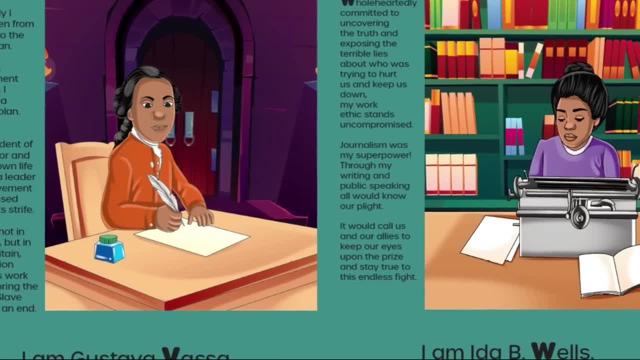 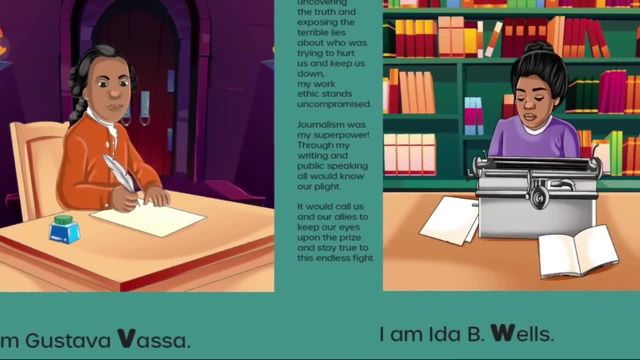 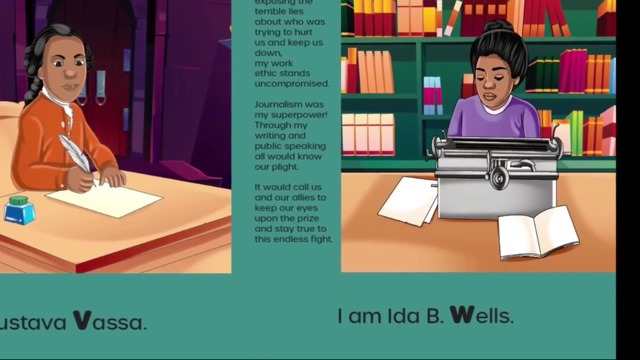 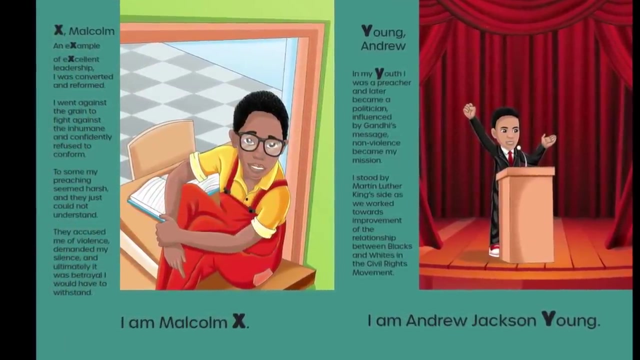 uncompromised journalism was my superpower, though my writing and public speaking. all would know our plight. it will call us and our allies to keep our eyes upon the prize and stay true to this endless fight. i am ida b wells, malcolm x, an example of excellence leadership. i was converted and reformed.